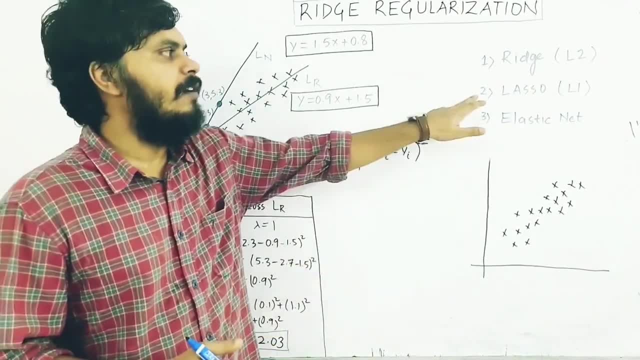 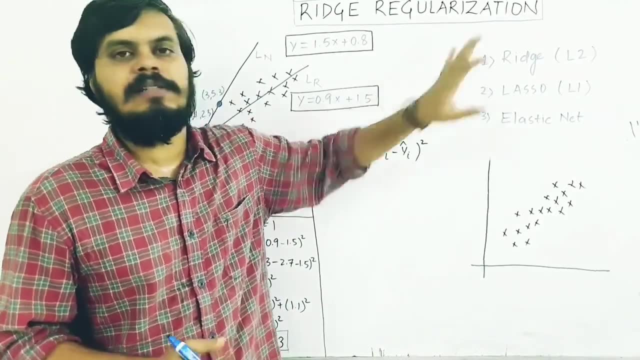 we also call this as L2 regularization. okay. the second one is lasso, and we also call this L1 regularization. and the third one is elastic length, which is basically a combination of ridge plus lasso. so in this video, what we are going to do is we are going to learn ridge. 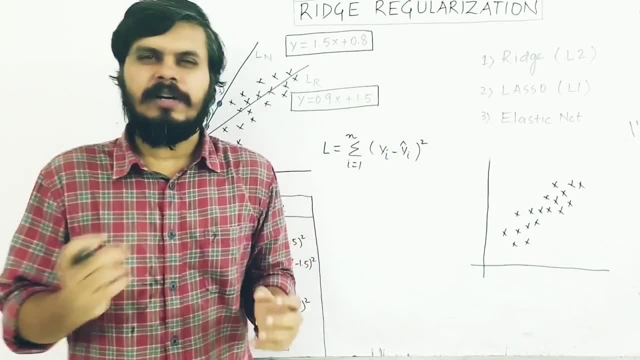 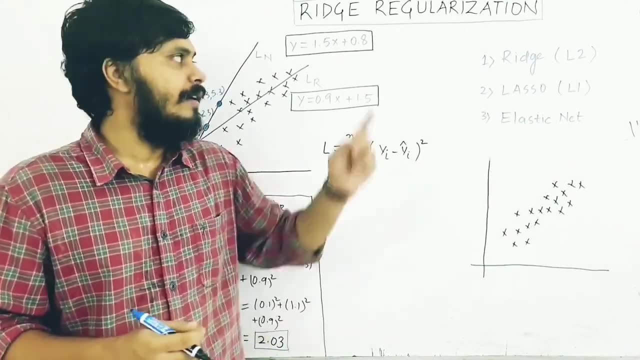 regularization. okay, so the setup of the video will be like this. it can be a little big, but we will. initially we will look at the whole geometry, intuition of ridge regularization on this code. then what we will do is we will apply code on a small toy data set. 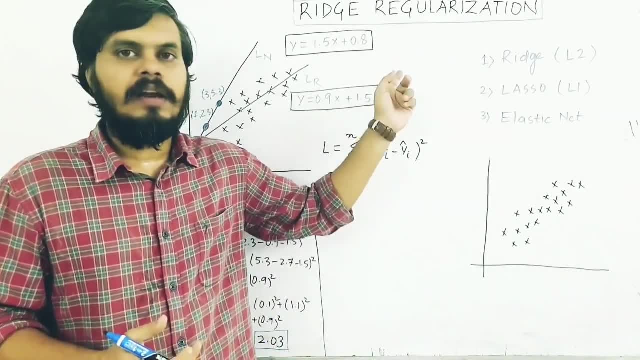 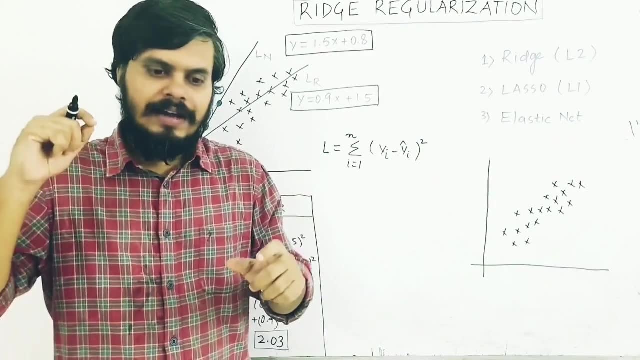 so there are built in classes in sklang to handle this. we will use that. and finally, in the third part of the video, what we will do is we will actually plot certain graphs and we will prove through graphs that, by using regularization, your overfitting is working. 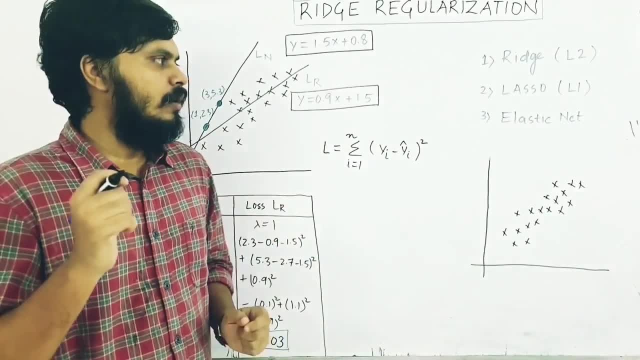 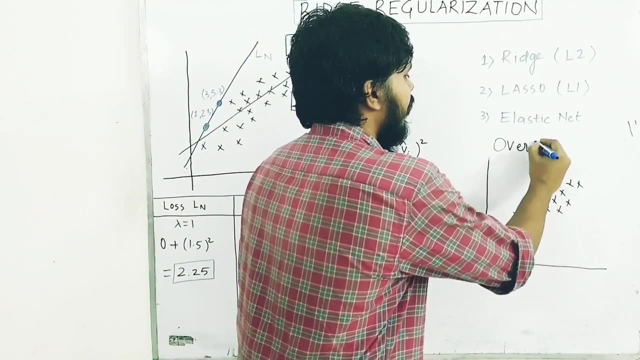 so that is the entire flow, so let's start with the video. so before starting the regularization part, I would like to discuss this term: overfitting. we have seen this term many times and it is like a very famous thing in machine learning. overfitting is talked about everywhere. 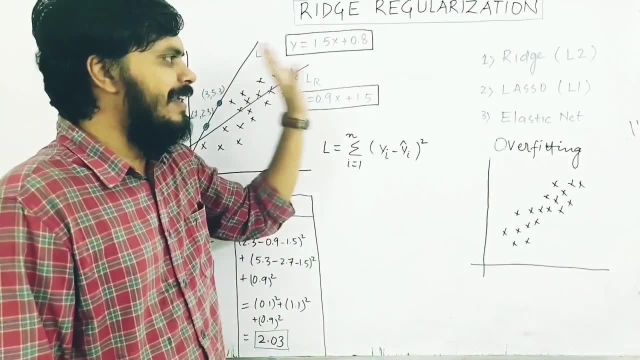 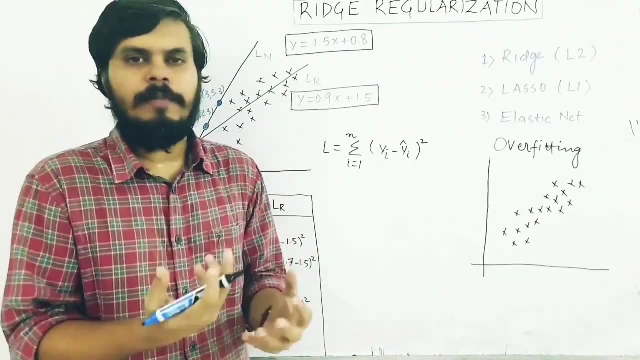 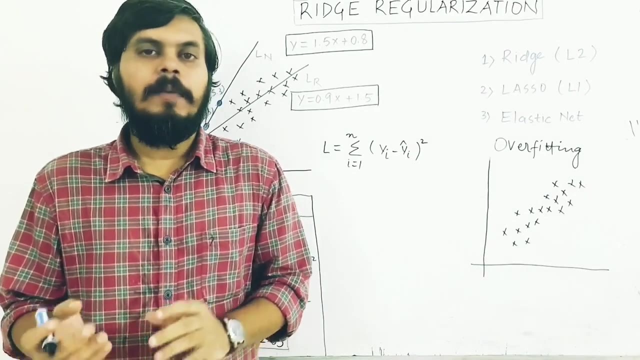 I am talking specific to this linear regression model- that what is overfitting. so, in general, if you talk about overfitting, then overfitting is this phenomenon, this criteria, where a machine learning model is performing exceptionally well on training data, but not so well on the testing data. 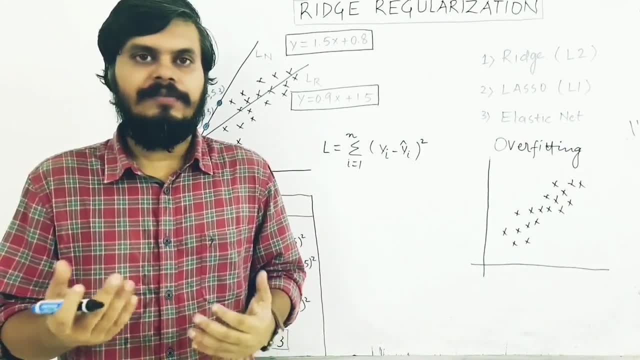 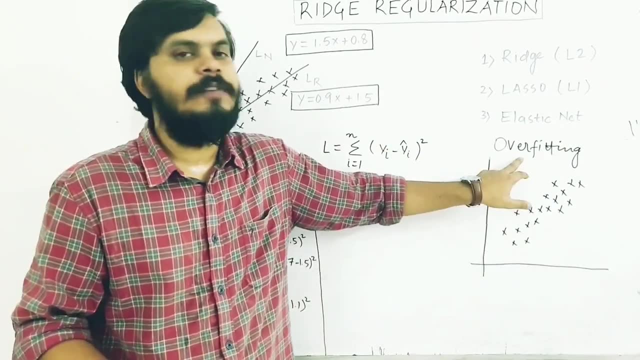 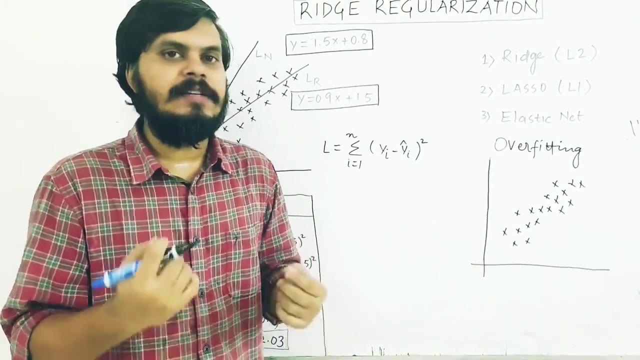 this means there is a lot of variance in your model. variance means its performance on one data set and its performance on a different data set is giving completely different results, and that is what overfitting is. this is the general understanding of overfitting. now let's see in the case of linear regression, what exactly does it mean? 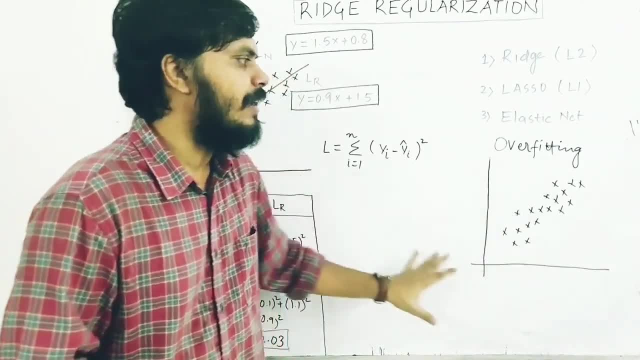 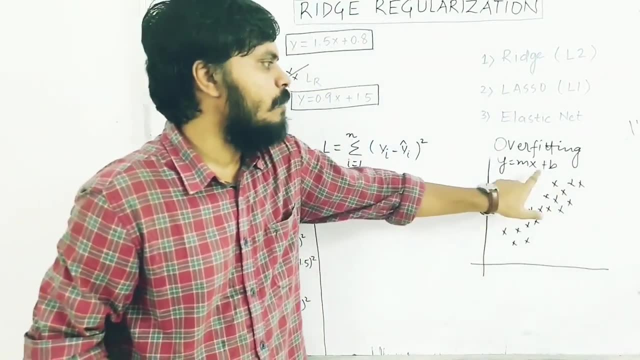 so look carefully. so the whole idea of linear regression is to find out the best fit line. y is equal to mx plus b, and in this also we have to find out the value of m or b. m is slope and b is the y intercept. so the idea is this, guys. 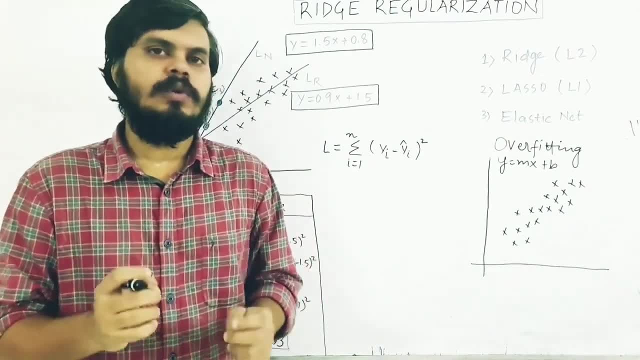 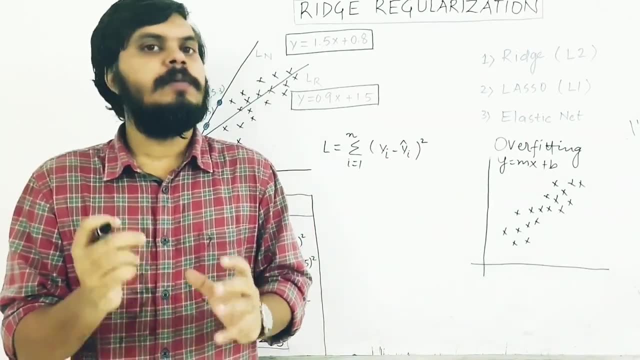 and you will see in future also when we will do all this in code. so you would notice that if there is overfitting in a system, if a machine learning model is overfitting, so if you want to know this directly, then how will you know? 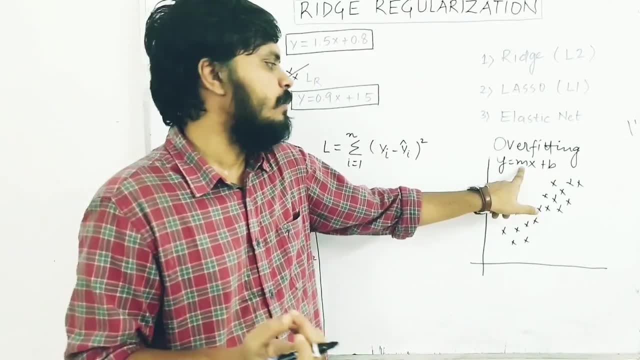 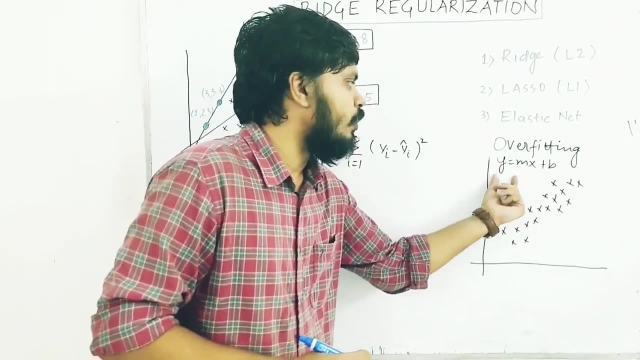 by finding out that. what is the value of m? you can also call it coefficient. what is the value of this coefficient? what is the value of this coefficient? what is the value of this coefficient? we have discussed this. this coefficient tells us exactly that. how much weightage will be there in finding out y? 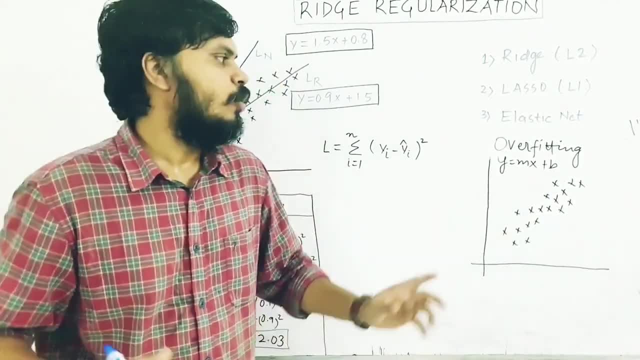 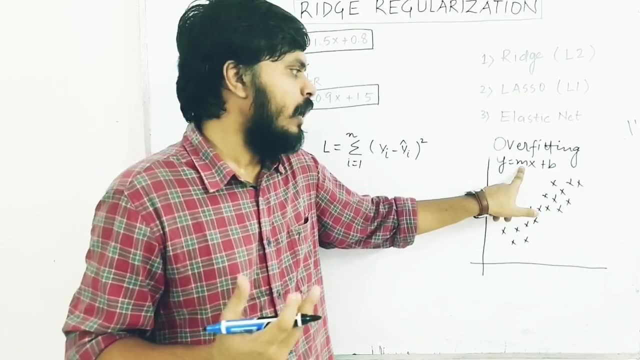 it means if the value of m is very high. so this means that in finding out y, the importance of x is very high, and if the value of m is very low, then according to your machine learning model, there is not much say of x in calculating y. 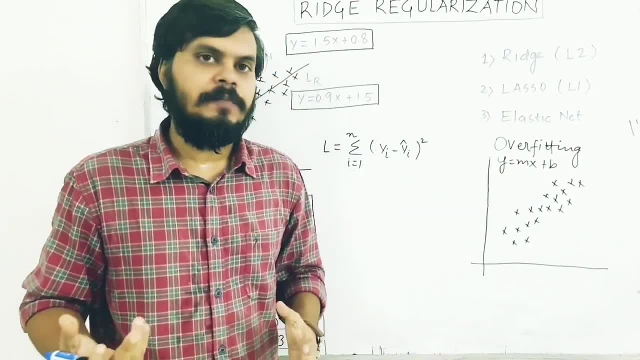 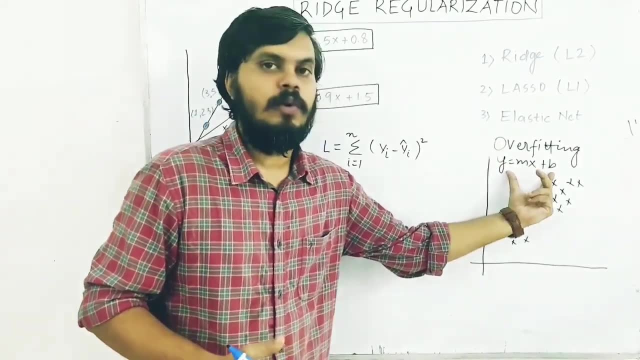 so this coefficient- you can also call it weight- it has a lot of importance and you will notice every time that whenever you will see an overfitting system, you will see an overfitted model, you will see an overfitted line segment there. this m. 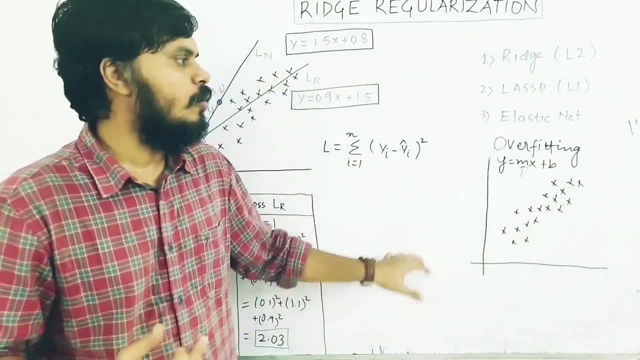 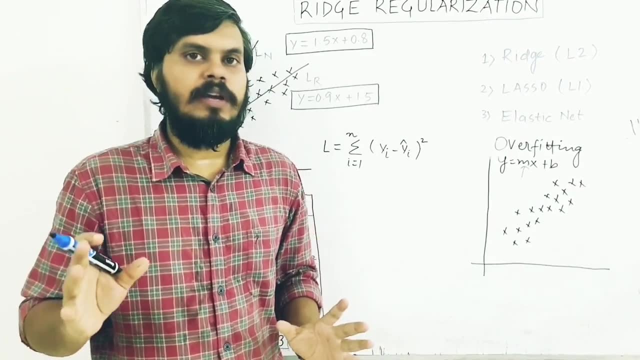 this m will have a very high value. so I am just saying that if you talk about overfitting in terms of linear regression, then it means that the value of this m is extremely high, and if the value of m is very low, then it is underfitting. 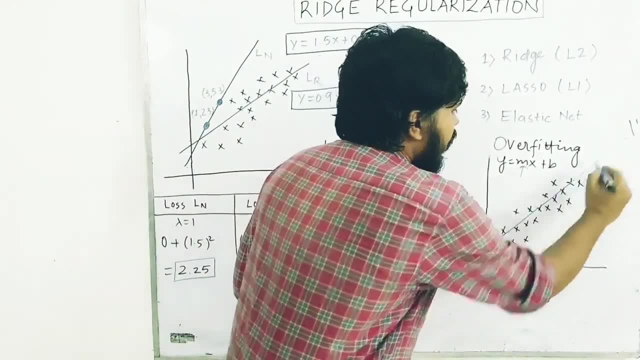 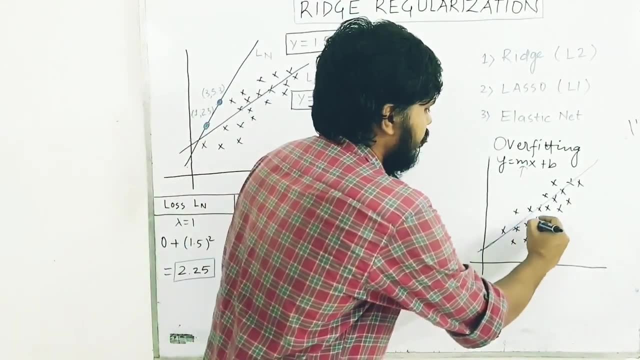 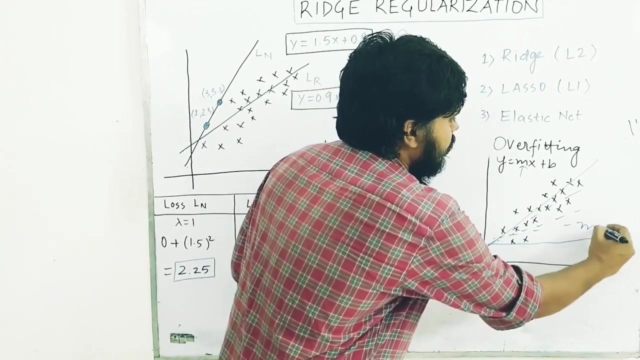 see, here we have data points. this is a correct line segment. this could act as a best fit line, but if you start decreasing its slope slowly, if you start decreasing its slope, then eventually you will reach a point where m would be 0, so y would be simply b. 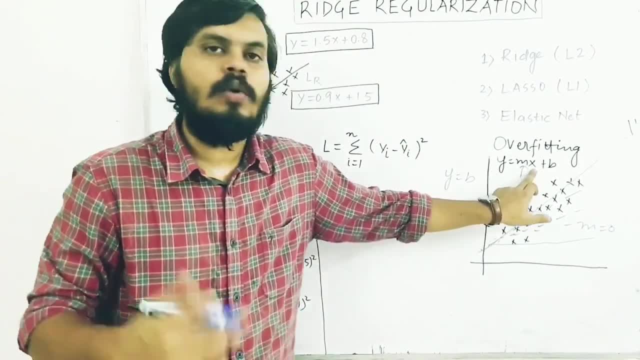 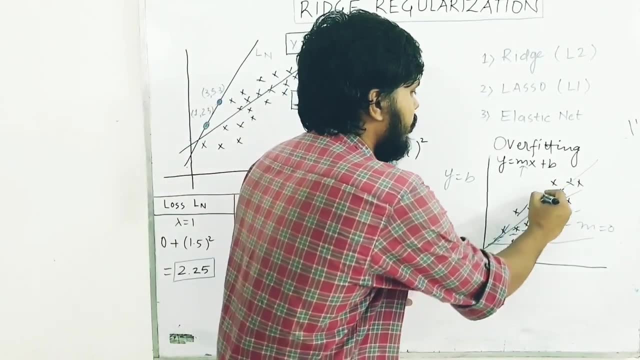 it means there is no need of x in calculating y. you just have to depend on x, and this is underfitting your system is underfitting right now. the second condition is that you start increasing the slope. you start increasing the slope and by doing this, you parallelize y with x. 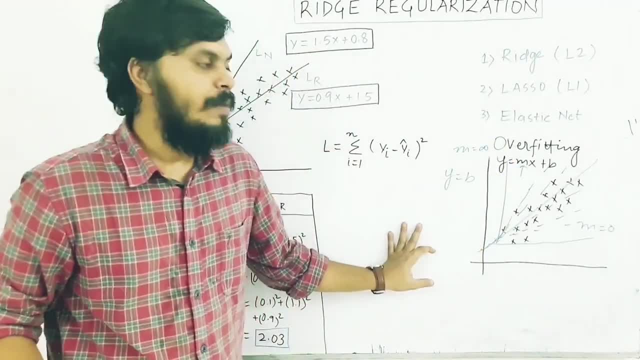 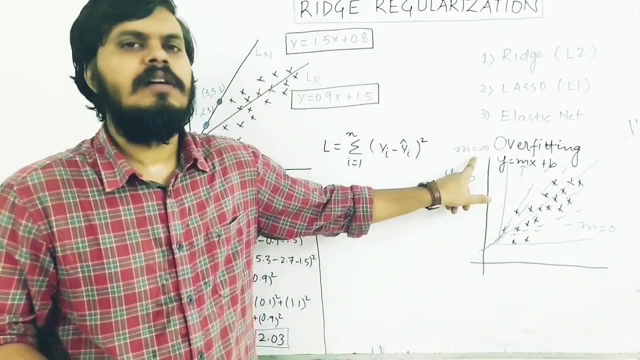 now m would be infinite. in this case it means to calculate y. the importance of x is the most important and there is no need to consider other things. obviously it will not be infinite. it is not possible, but a very high value is telling us that to predict y 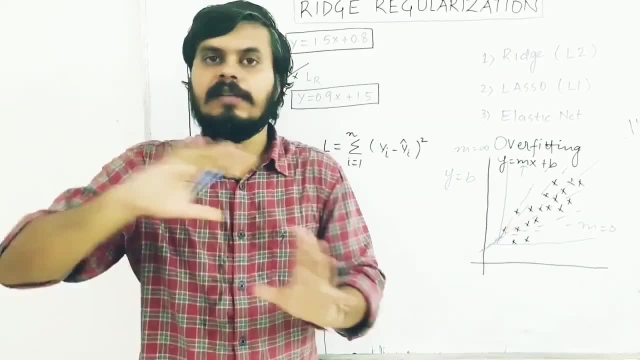 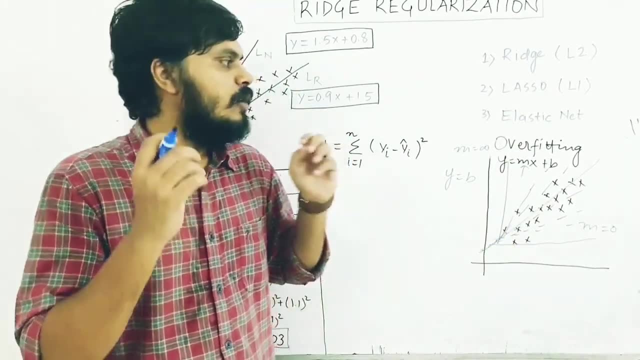 m has a very high weightage and your system will forget everything else and will only focus on x because its coefficient is very high. so this is what overfitting is. so this means, if you want to reduce this, if you want to reduce overfitting, 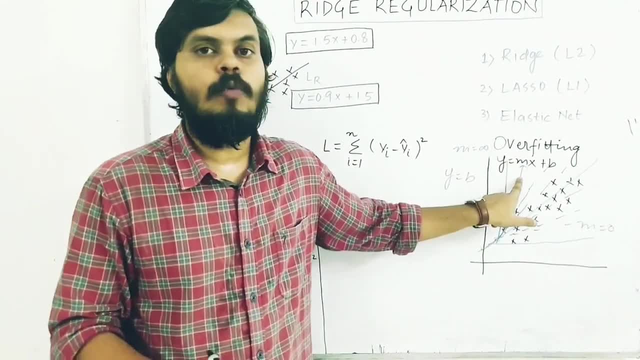 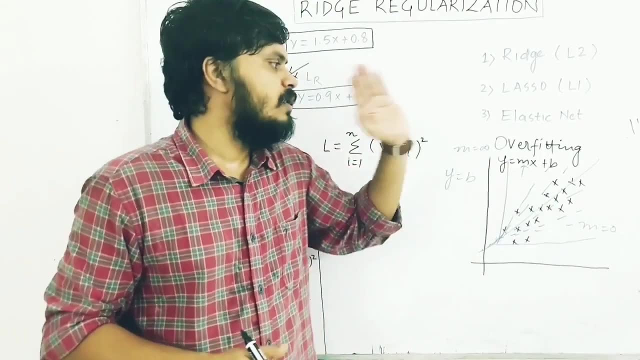 then mathematically it has only one meaning: that you are decreasing the slope in any way. right means you are taking a little less than what you have, not too much. if you take too much then it can be underfitting, but you have to take a little less than what you have. 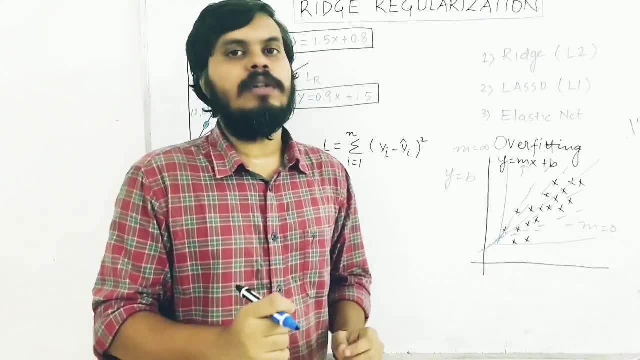 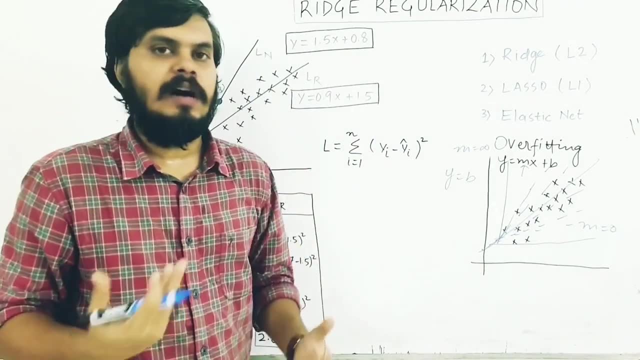 so if this understanding is developed, then we can understand very well what is regularization. so look carefully. let me explain the whole setup once, and then I will do it and show you how this thing is working. so this is the setup. here there are two types of points. 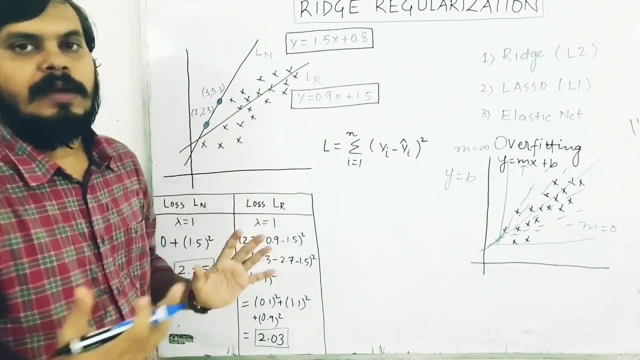 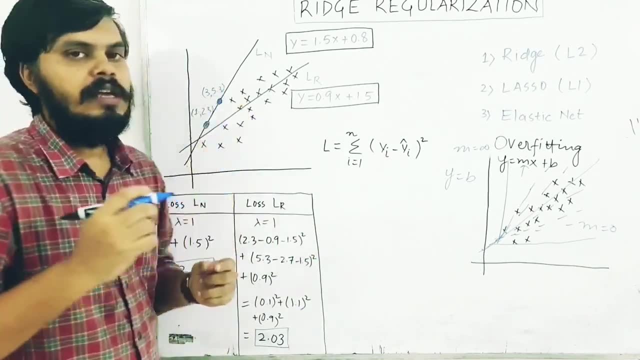 so this is my data set and here there are two types of points. so one set is training and the second set is test. so these two points are the points in blue colour. these two points are actually the training points. so there are only two points in our training data. 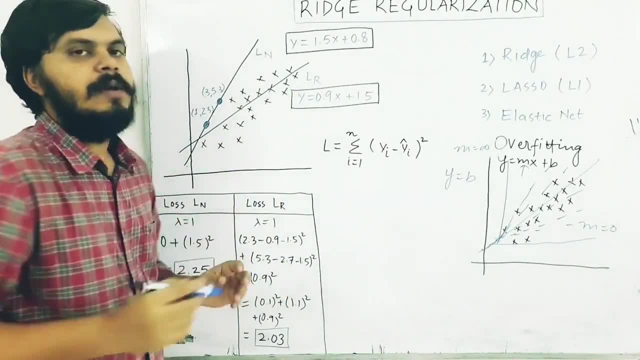 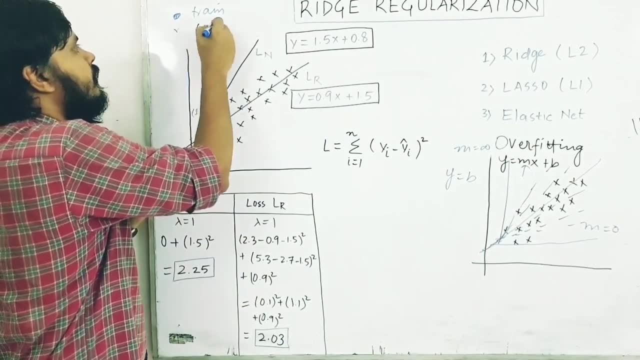 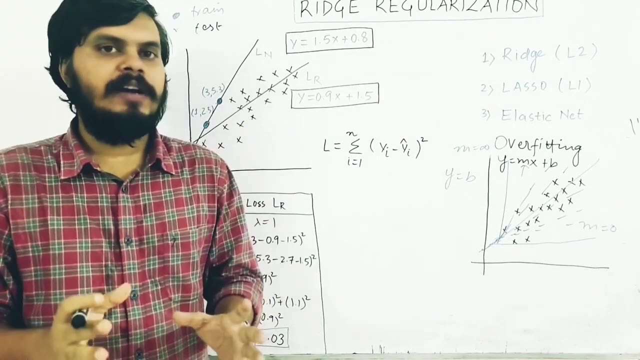 there are no more points. right, and the rest of the data is my test data. ok, so this thing is train and this thing is test data. ok now. now think for yourself: if you train your model on the training data, then you have to find the best fit line. 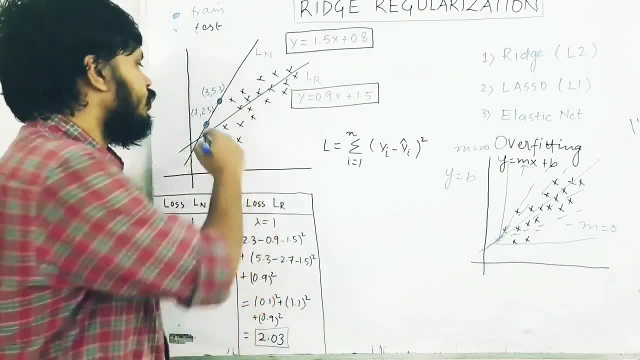 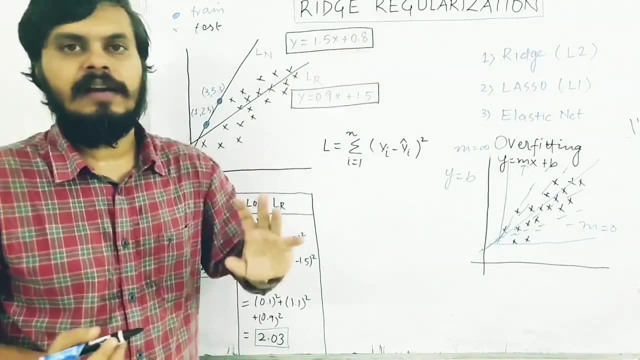 and if you have only two points, then the best fit line will be the same which will pass from both right. so I have already calculated this line. this is that line y is equal to 1.5x plus 0.8 simple coordinate geometry. I have calculated the slope from these two. 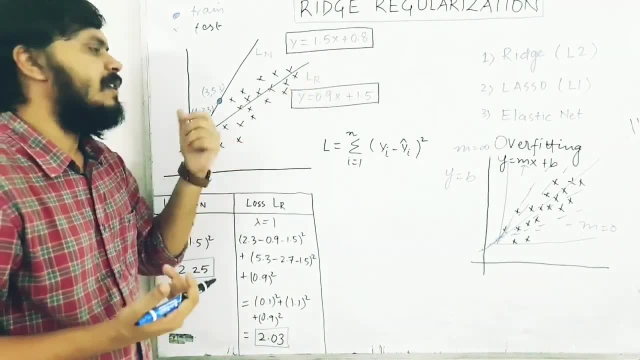 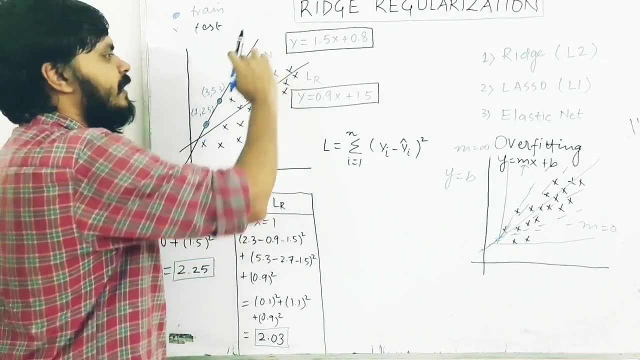 I have put this one point in this equation: y is equal to mx plus c, and I have calculated b and this is the equation of the line. ok, so this is my best fit line, right, this is my best fit line, and see for yourself. you can understand that. 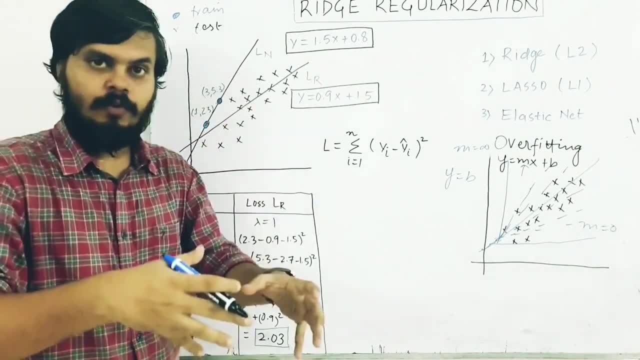 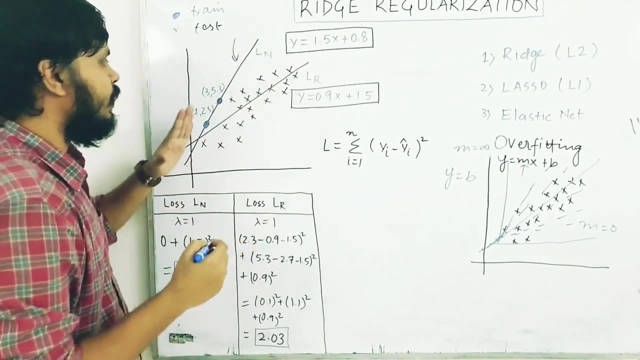 because I had so little data that my line is focusing on these two points only the pattern in the actual data. I could not pick it and it is clearly visible that this is the case of overfitting because my training line is going somewhere else but my actual line. 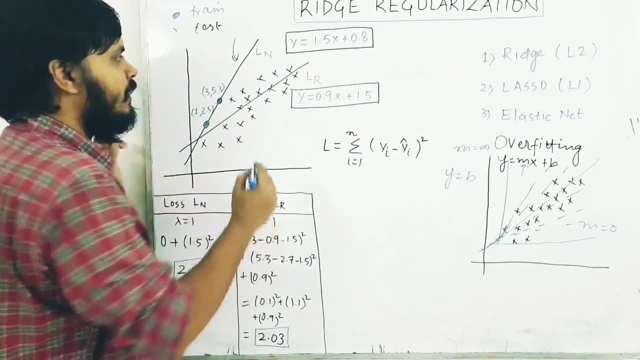 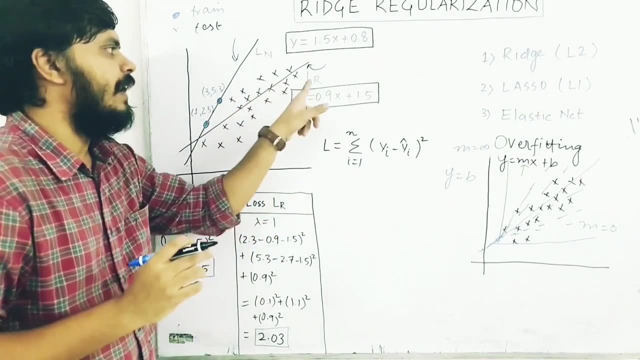 should have been something else. right, this is already visible and let's consider this that hypothetical line which may perform better than this line, although this line, the second line, LR, will make more mistakes in the training data, but still it will perform better in the test data in comparison to. 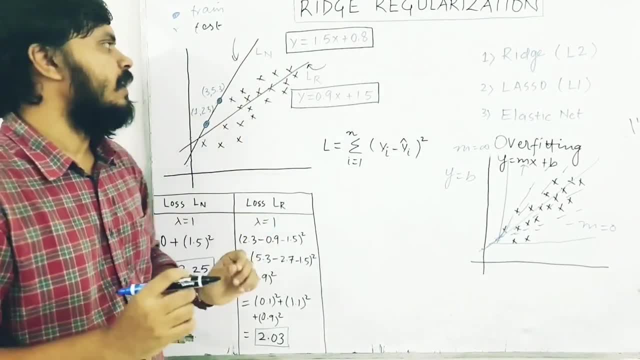 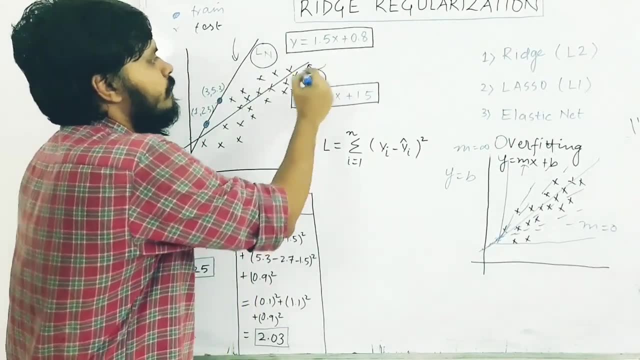 this line LN, right. so now what I have to do? somehow I have to convince my machine learning model that don't choose this line, choose this one, right. this is my goal, and how will I do this? we have to see this in regularization, ok, so watch carefully. 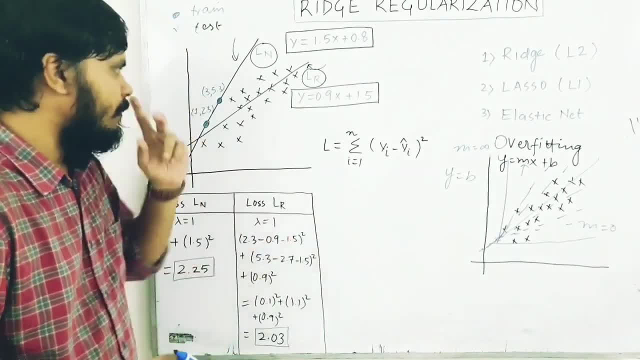 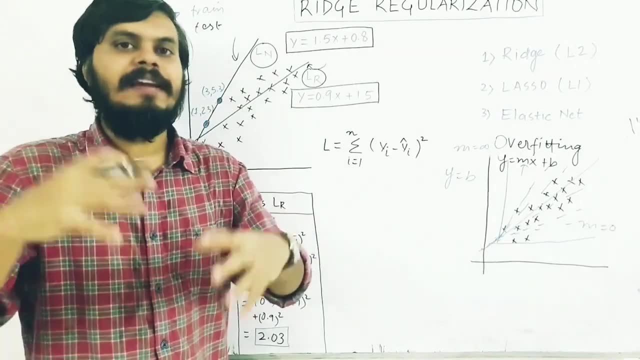 how do we select lines? you already know this. so what you have to do, you have to minimize this error right: the actual value and the predicted value, the squared sum. you have to minimize its magnitude, its value right, and in that you had seen two techniques: OLS. 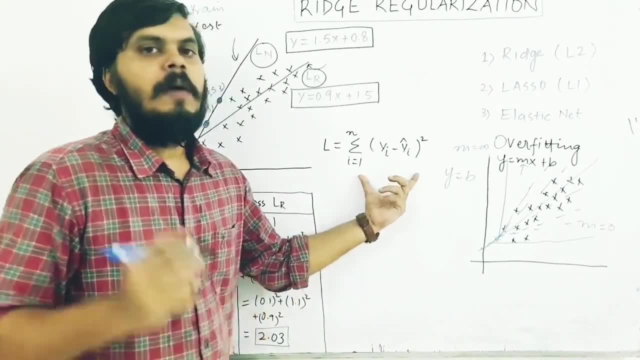 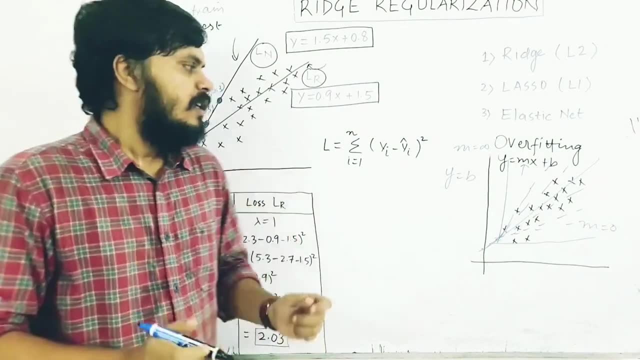 gradient descent, right. so the whole idea is to minimize this term. what you do in regularization, you just add an extra term which we had studied in the definition of regularization. Q adds an extra thing. so that extra thing is actually this. let me write it down: lambda M. 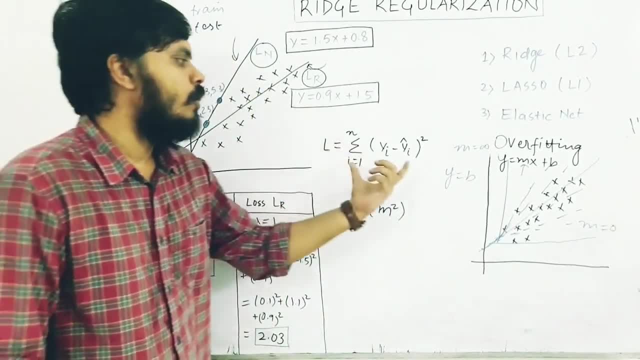 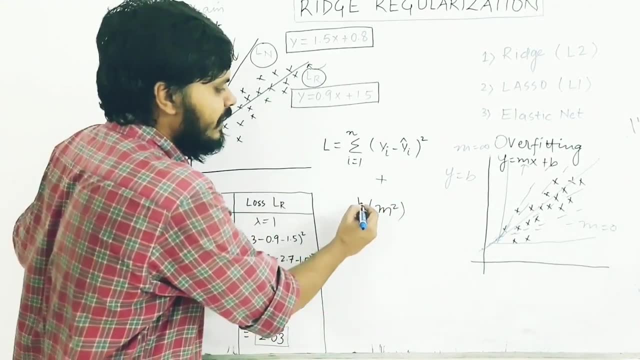 square. so now you are saying that my loss function will not only be this, but in that your term will also be added right. and what is this term? this lambda is actually a hyperparameter. this is a hyperparameter. its value of Q is: you can tune its value. 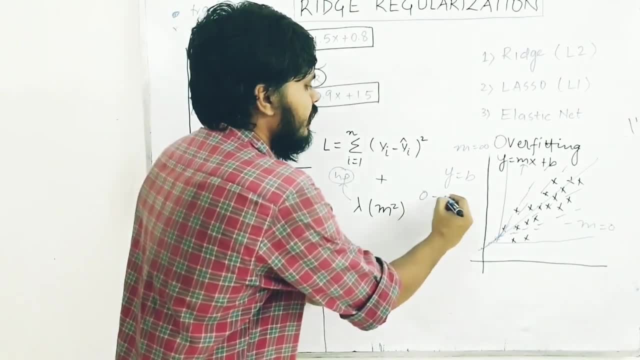 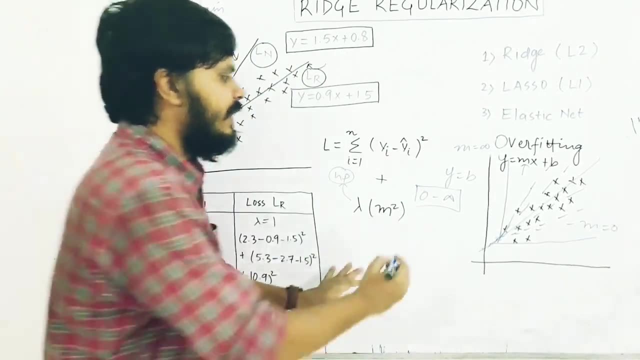 up and down. generally, its value is from zero to infinity right? so this is lambda. you will tune its value and this is M. M is basically your slope, this is your slope, right? and guys, now let us see that. just by adding this term, how will I convince? 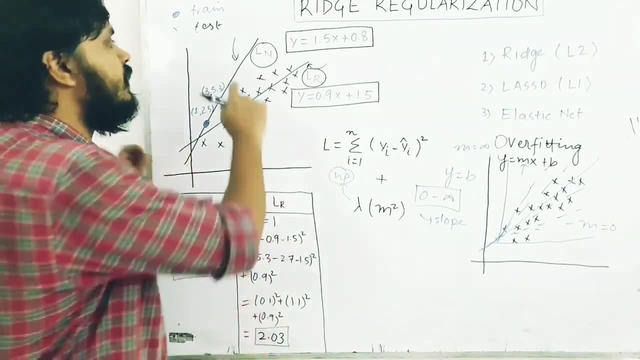 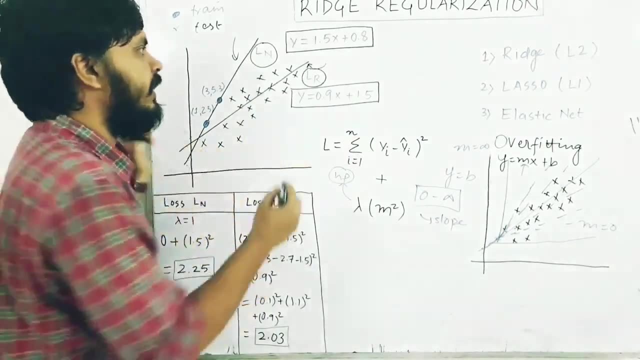 my machine learning model not to leave this line and leave this line right. by the way, this is the equation of the second line and this is just hypothetical means. I have just chosen this first. I have chosen that I want slope less, so I have 1.5. 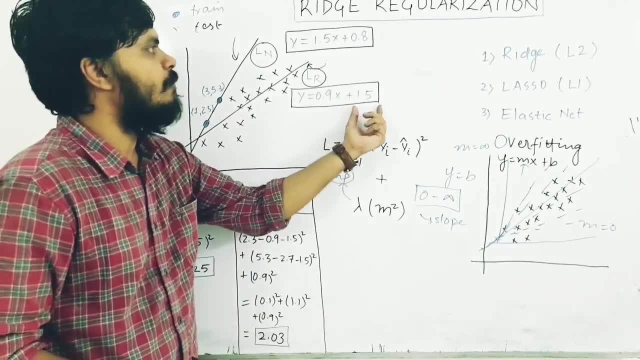 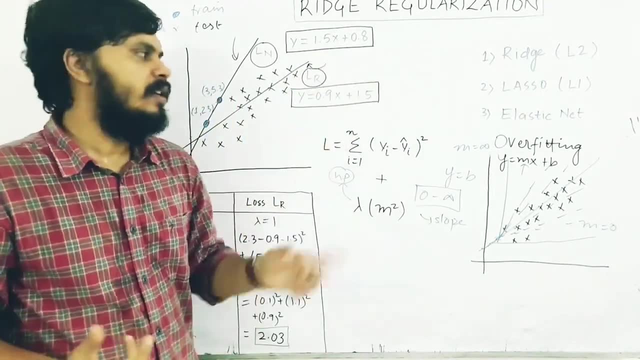 so I have this 1.9, okay, and obviously if I'm tilting then its intercept is increased, so its 1.5, its 0.8, this cycle, like this is. this is actual in these 2 points. this is actual. this is like: 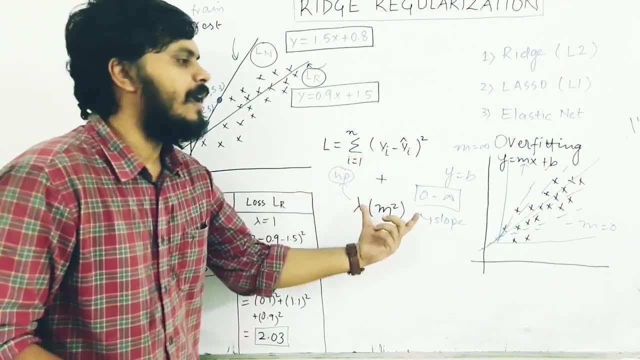 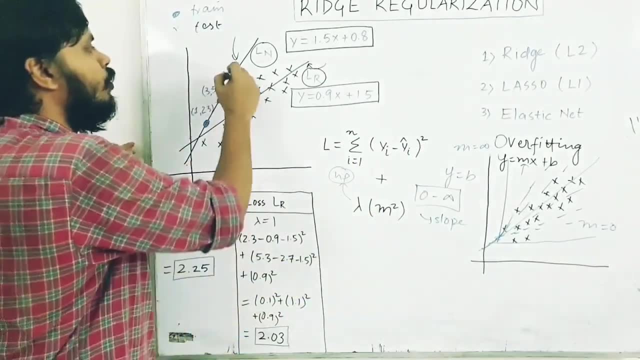 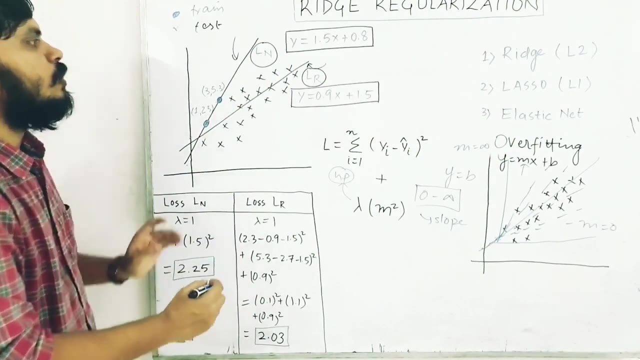 my assumption that this line can be okay. so now what I have to do? I I have to value. I will calculate for both of these lines. so let's calculate it for the first line, Lm. I have calculated it here. let's see once. so it has two components. first, how much Lm. 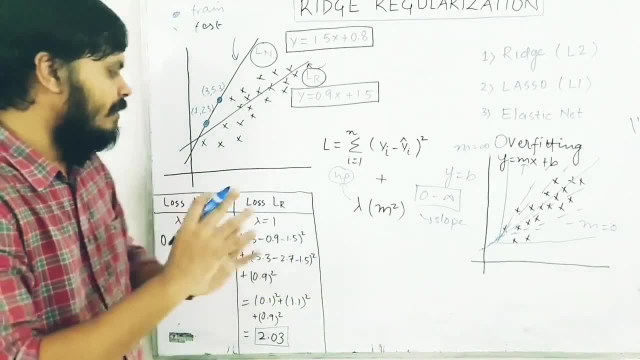 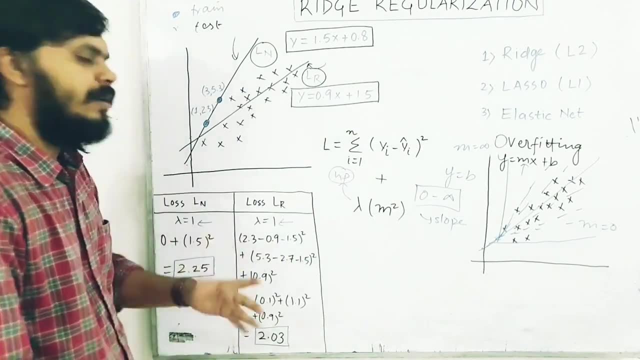 is coming on residual and second, lambda multiplied by m square. one more thing: we have taken the value of lambda for both the lines as 1, so that both are same. you can tune it. but we have taken lambda equal to 1, now you can easily see that if this line is passing. 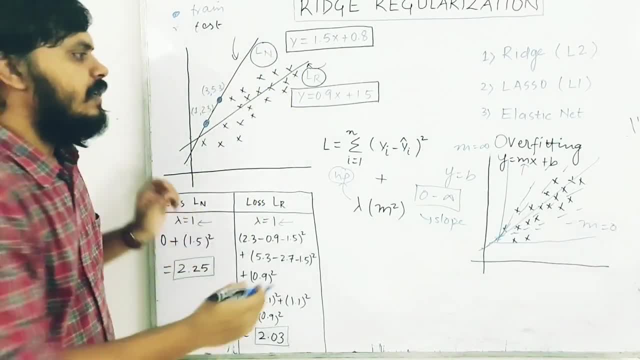 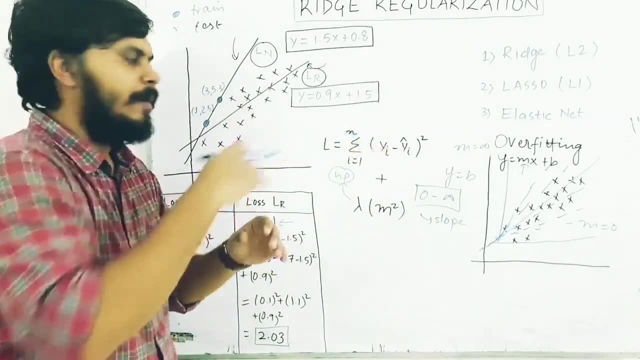 from both the points, then obviously this term would also be 0,. right, because y predicted and y actual has no difference at all for both of the points you are passing from above, so this term will become 0, right now let's talk about this term. this is equal to 1, and 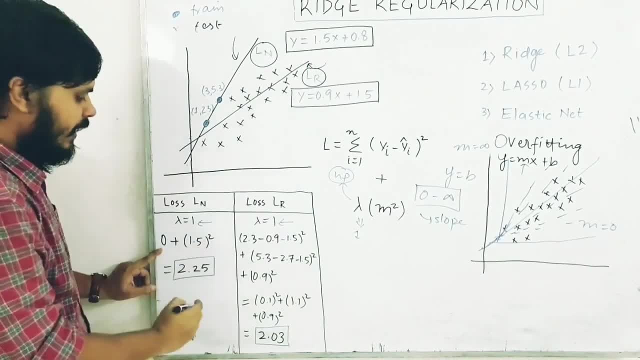 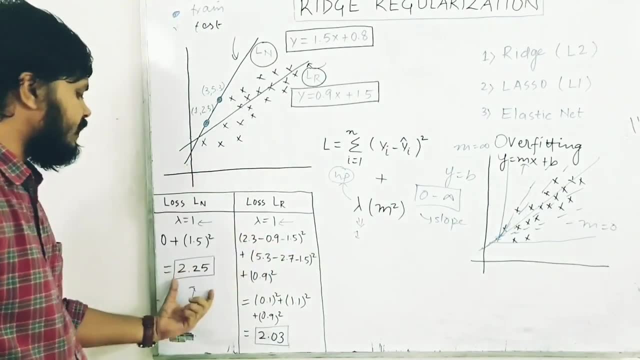 m, for this one is 1.5, so I have squared it to 1.5 and this is the loss. so, on this screening data, after adding the term of regularization, my loss is 2.25, so my machine learning got. 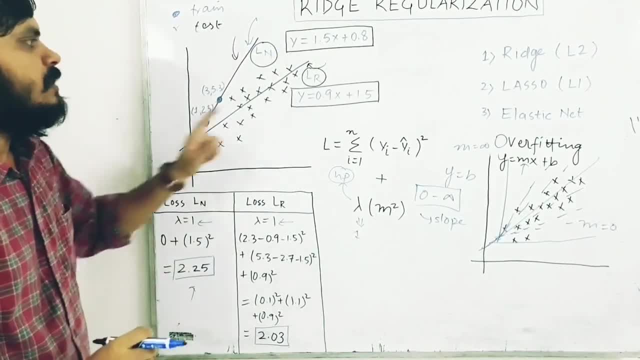 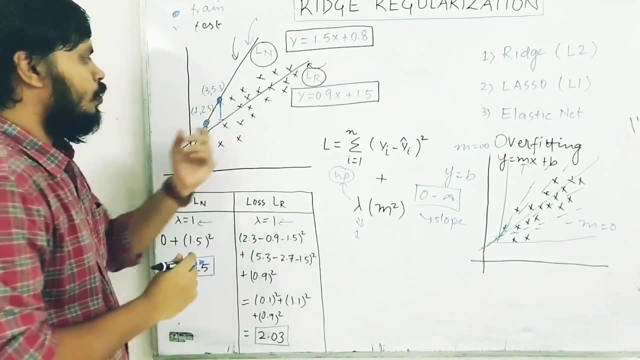 the value of 1 and y and I have to face so much loss for this line right now. let's talk about the second line. now, the second line is making a mistake. see, this is the mistake. it is not passing it, so it is making a mistake right now, if you have to calculate, 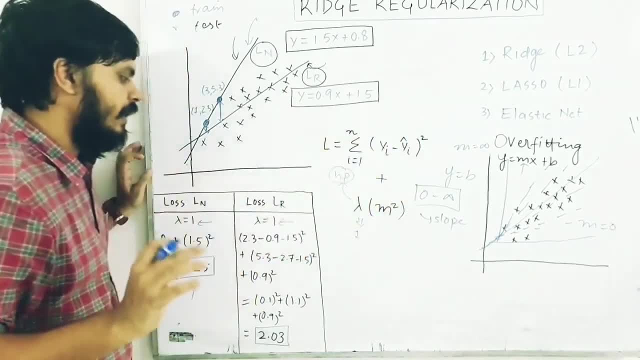 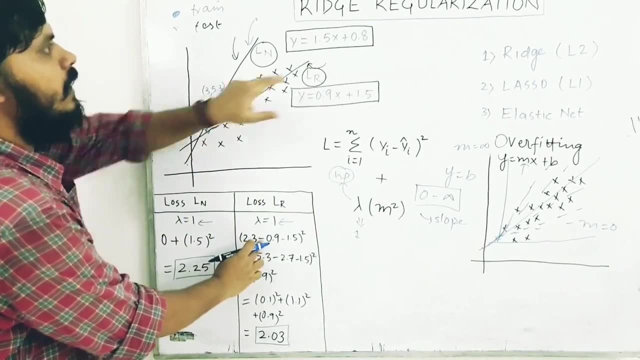 this then, basically, you have to get the 1st point's predicted value plus square plus the 2nd point's predicted value squared right. so you can see, I have simply plugged in. so I have written 2.3, this is the term of my y minus in this equation I have given. 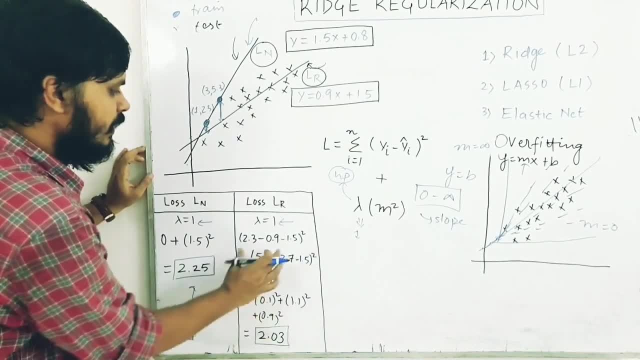 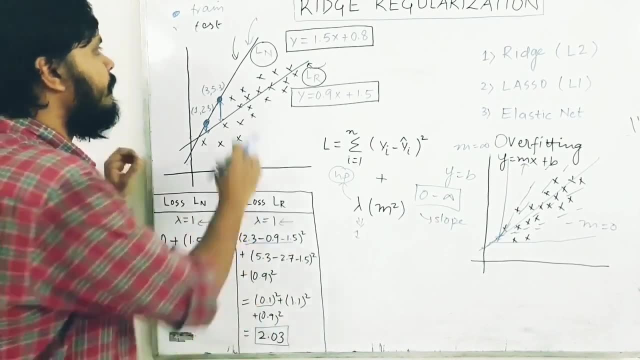 minus 0.9 plus 1.5. so minus 0.9 minus 1.5. when you solve this term, then you get 0.1 square. this is the loss of first point. now the loss of second point is 5.3 minus 0.9 multiplied. 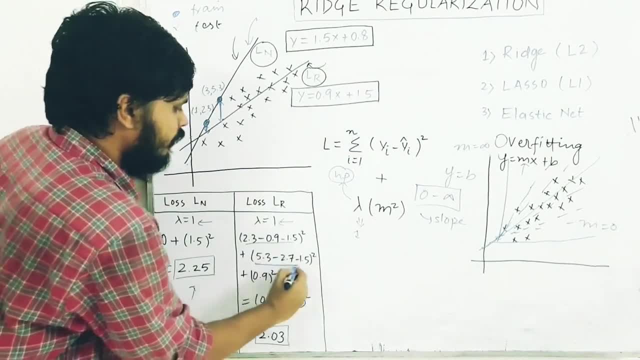 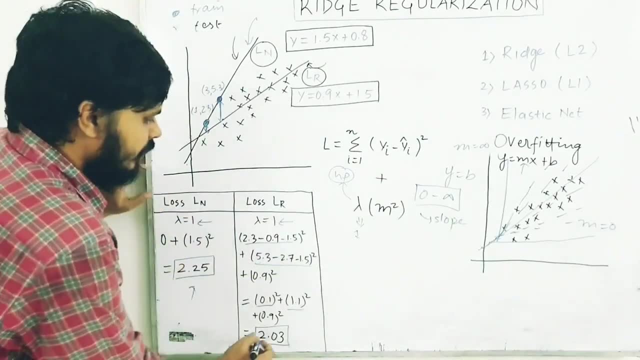 by 3, 2.7 minus 1.5. after solving this, I got 1.1 square. and lastly, I got lambda multiplied by n square. here n's value is 0.9, so I got 0.9 whole square. and as soon as I solved this, 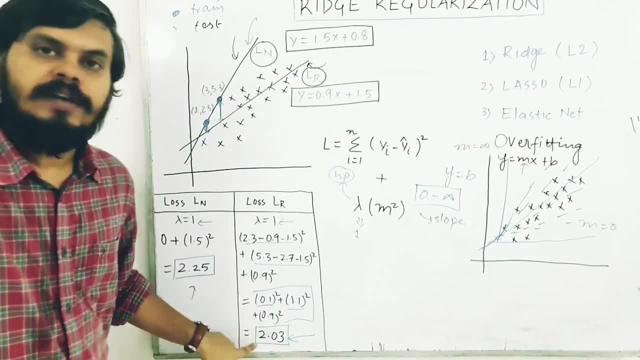 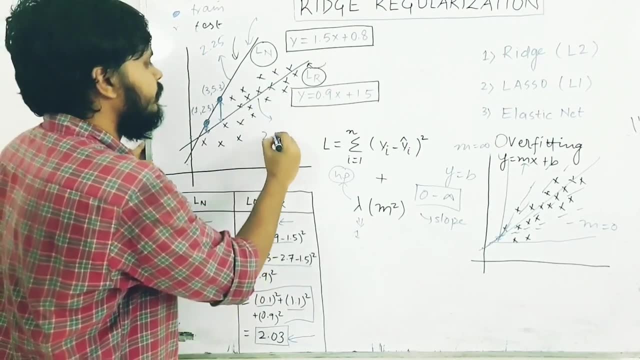 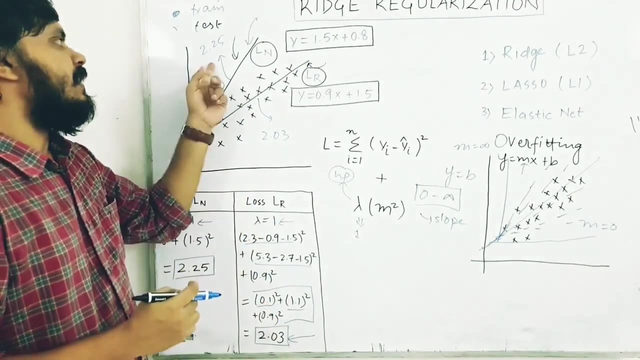 whole term. this is my loss for the second line: 2.03. so you can see, for this line it's 2.25 and for this line it's 2.03. now your machine learning model doesn't have any other option. it clearly shows that this line has more loss in comparison to this line. so obviously, 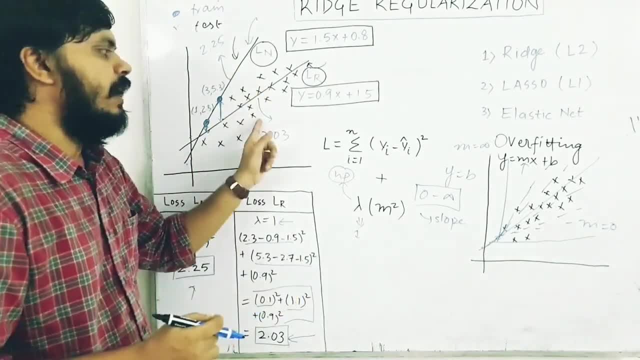 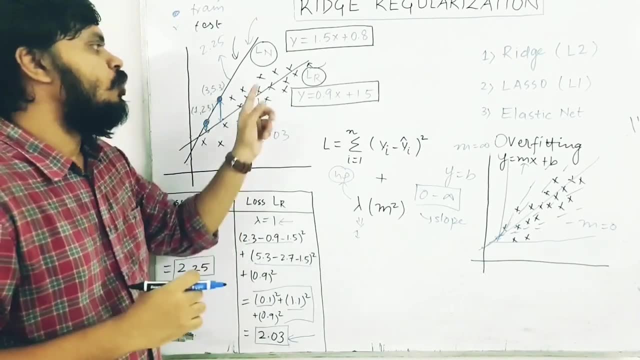 if you give it two options in between these two lines, then it will not be able to solve this problem. so: this line and this line. it will automatically choose this line, even though this line is making a mistake on the training data. still you will use this because 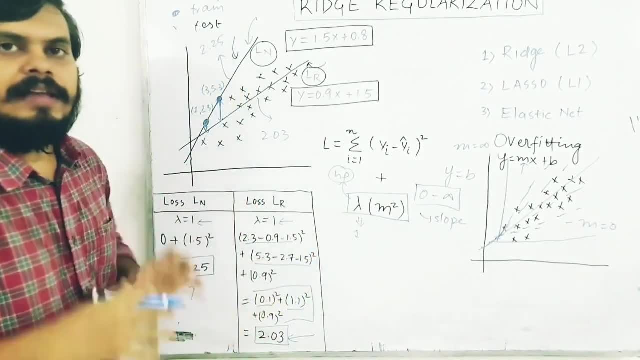 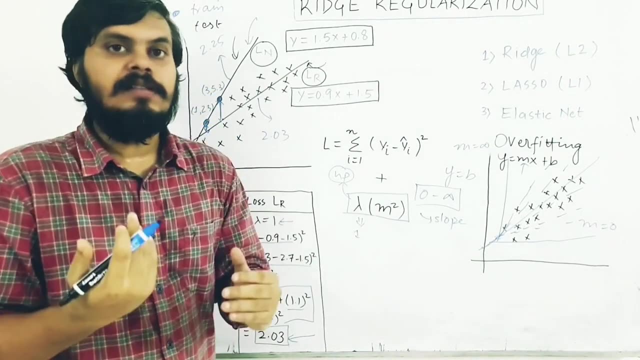 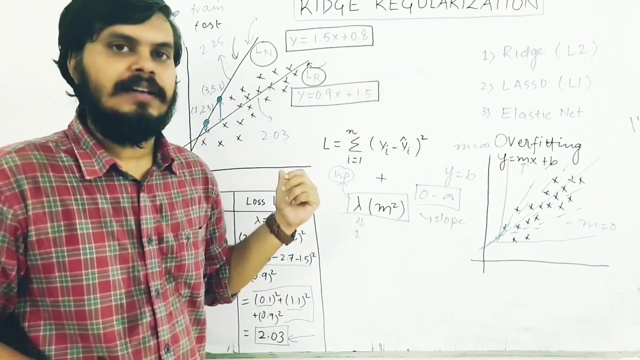 you added this down of regularization. I guess you are understanding this point, guys. so the whole idea was this: that, although your bias increased a little, but your variance significantly decreased- right, and that is the whole idea behind bias- variance paid off and regularization is doing exactly the same right. two things which are odd is good, and two things which 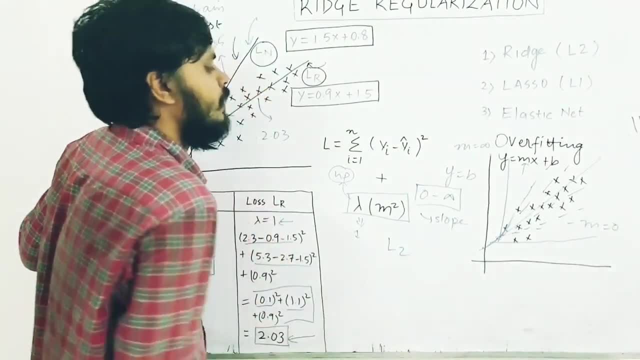 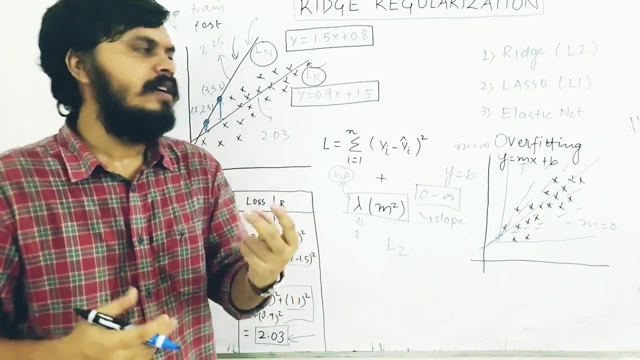 are good and two things which are bad. so the first thing is that, in fact, the reason why we are discussing this is because, first, why we call it L2 regularization? because, let's say, if you have another axis, if you have two input columns, then what you do is you do lambda. 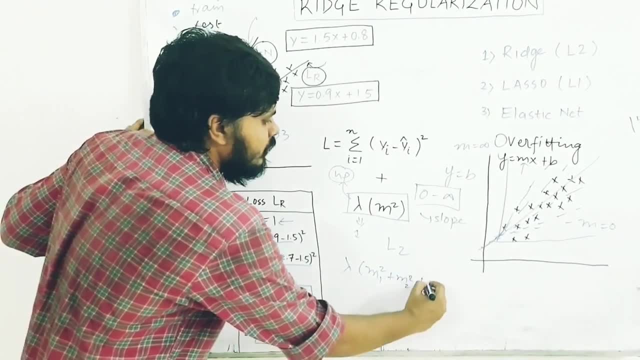 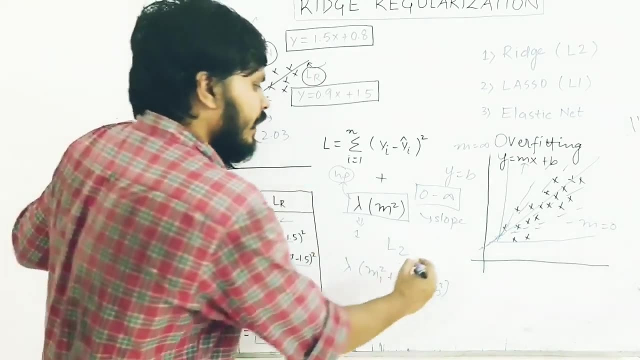 multiplied by M1 square plus M2 square. if there were one more, then it would be M3 square. so, basically, for every extra axis, the coefficient you have, you multiply it by square. so, since you are multiplying by square- that's why you are doing this- so you are multiplying it by. 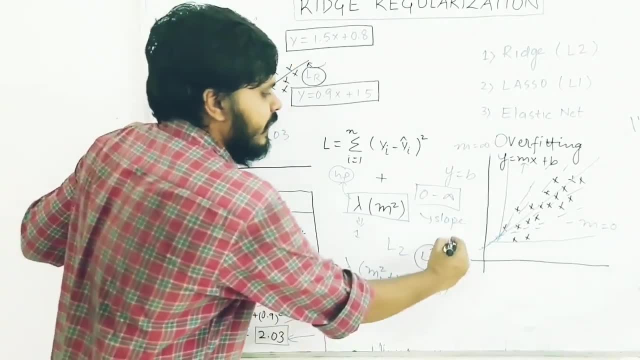 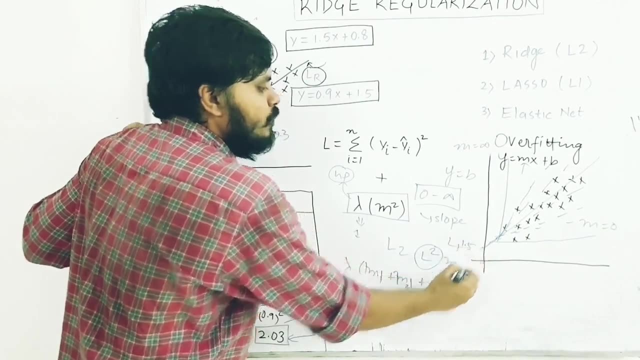 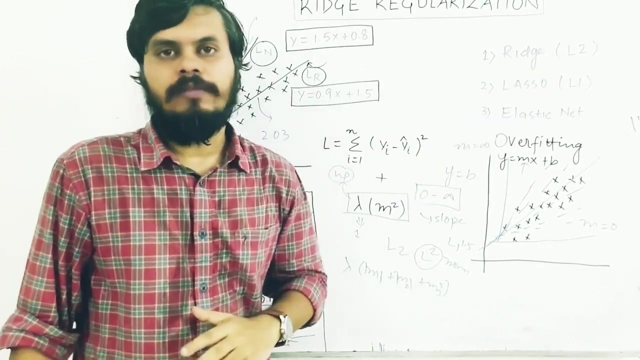 Similarly, there is L1 norm, which we will study in the last one. there you take only absolute value. Similarly, 1.5 norm can also be there. 2.5 norm can also be there. any norm can be there, But most famous is L2 norm and L1 norm square and absolute value. 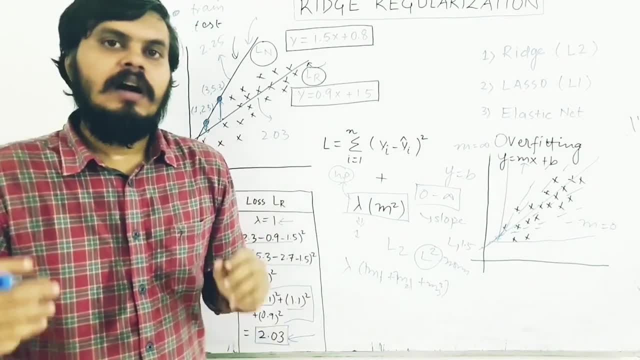 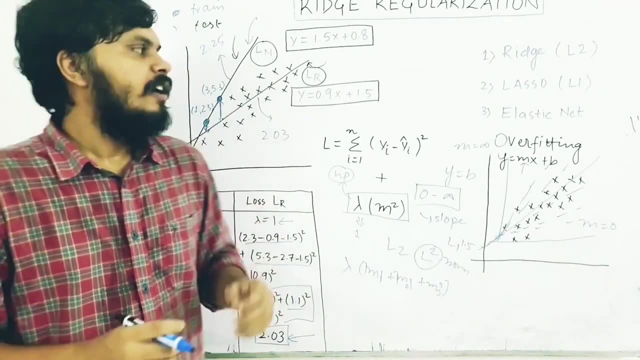 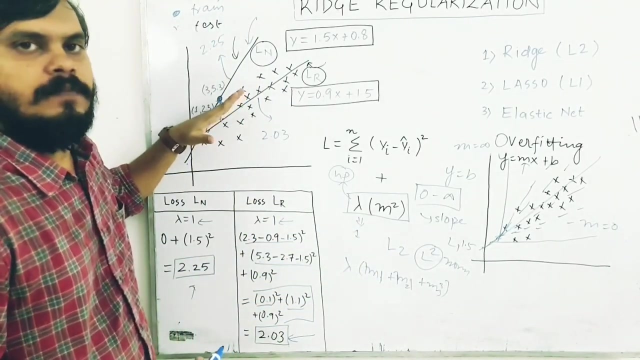 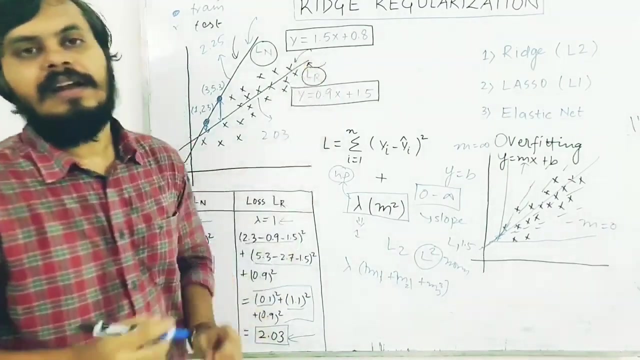 So, guys, I hope you understood this video till now, Because after this we are going to do the same thing in code. I will just summarize once: the whole idea behind regularization is To add this regularization term, which will reduce the slope of actual line, And your model will have to collect the other lines because the other line will give less error. 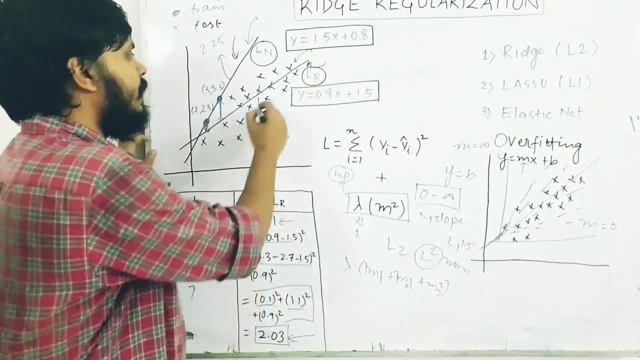 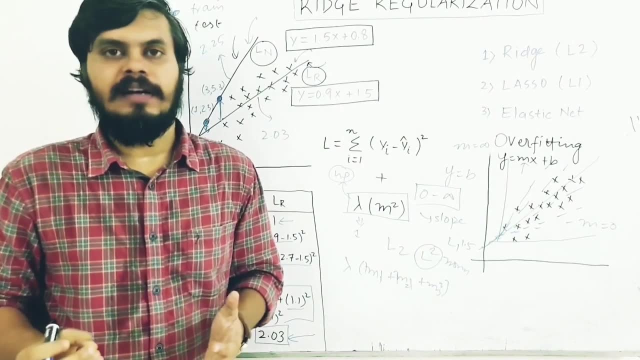 And because of this your bias will increase, because this line will give less error in training data, But your variance is decreasing. and you want exactly this: you want to reduce the overfitting, But if you will do it too much, then you can under fit it. 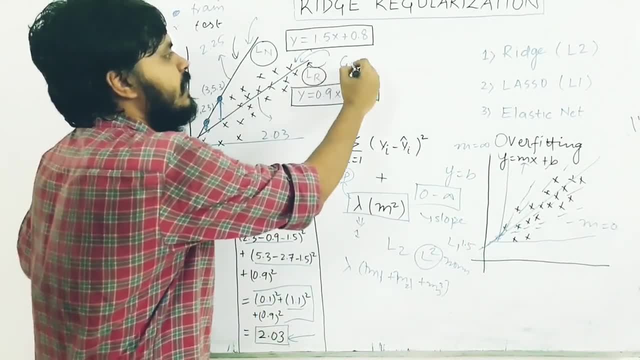 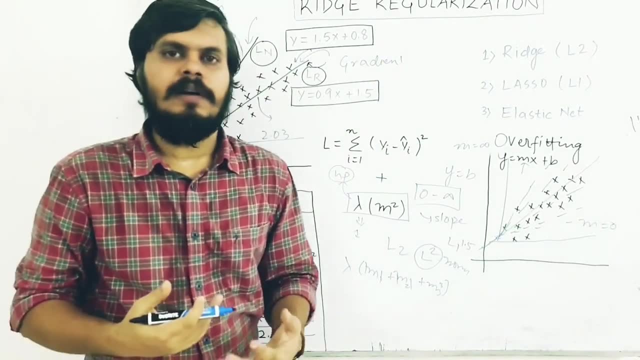 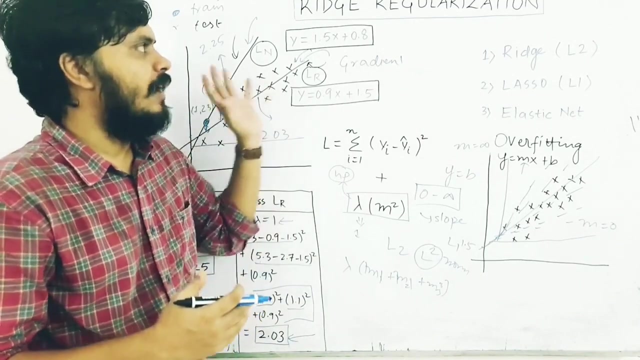 And obviously, to calculate this you use the gradient descent algorithm. It is not necessary that this line is the only line. it is possible that there is another line whose loss is less than this, So it is automatically calculated through optimization. So now that we are into this regularization thing and we understood how it works, 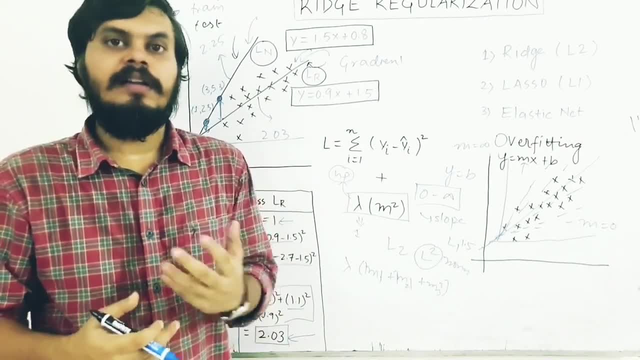 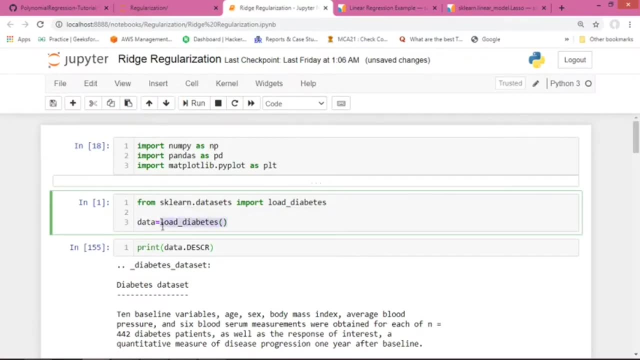 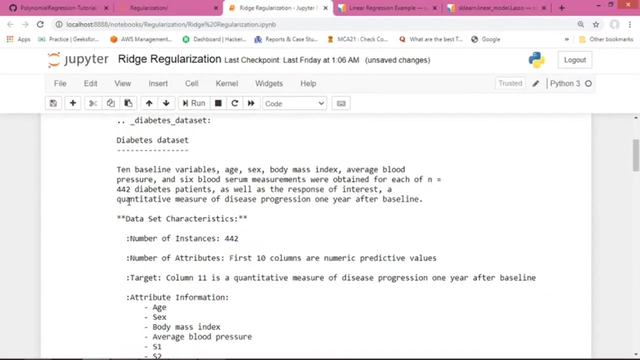 Let's dive into the coding part and let's see how it works in scikit-learn. I have picked up a simple data set. this is a part name with scikit-learn Called load diabetes, And this is the description of the data set. So actually there are 10 input columns. 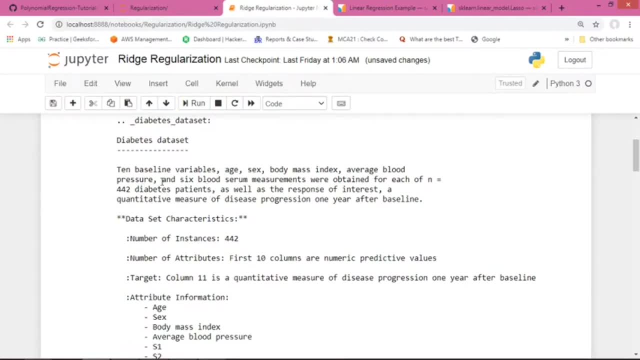 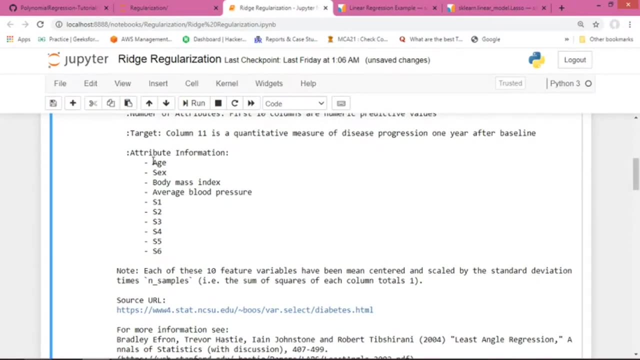 8, 6, body mass index, average blood pressure and 6 blood serum measurements. So in total there are 10 input columns And your target column, column 11, is a quantitative measure of disease progression One year after baseline. So that is a number which shows how much the diabetes has increased. 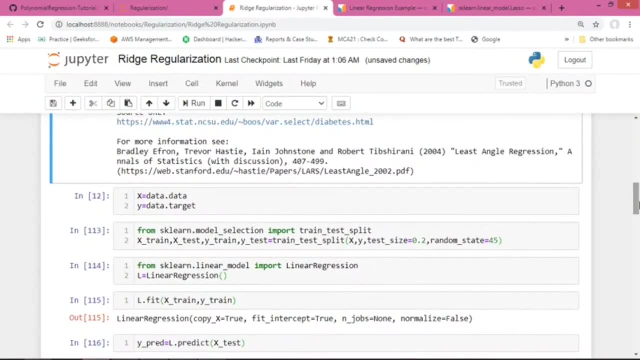 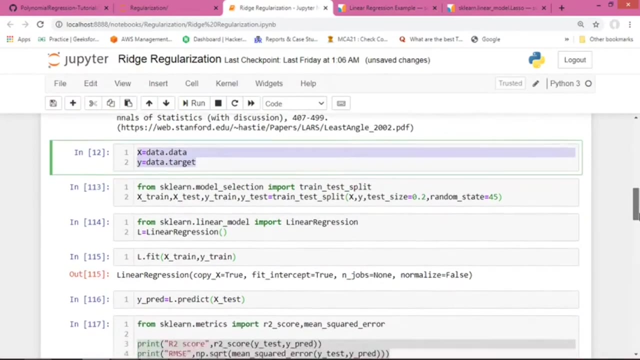 So what I have done is: first I have tried to solve this notebook with linear regression And I have measured R2 score, etc. And after that I have done the same thing with ridge regression. So here we have extracted our input and output. In this next step, we have split our train test. 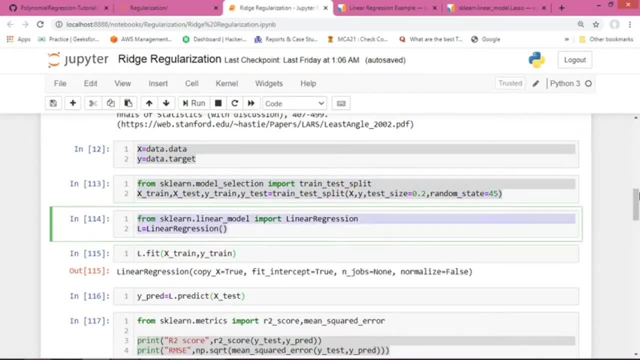 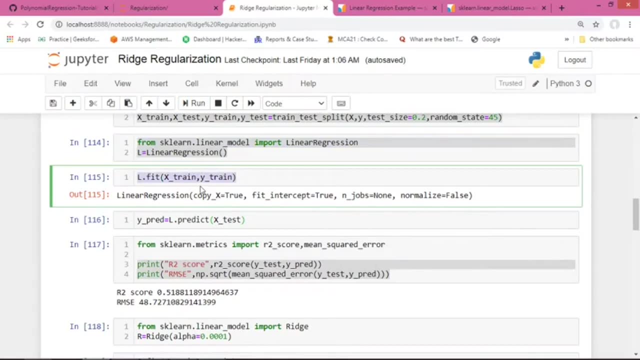 In this step, the object of linear regression, And here we have trained our model using the linear regression algorithm. And when it is trained, we have used the predict function to predict the test data And stored it in the wipe-read. And in this step I have measured the R2 score and the RMSE score. 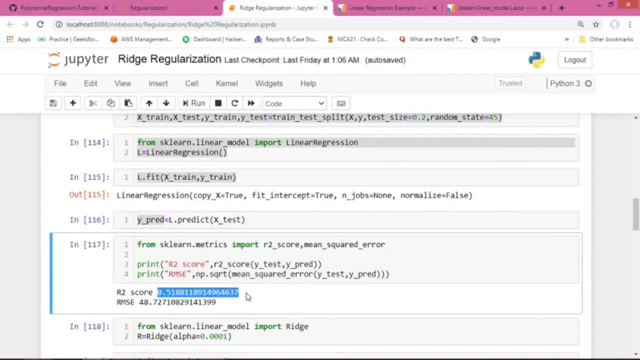 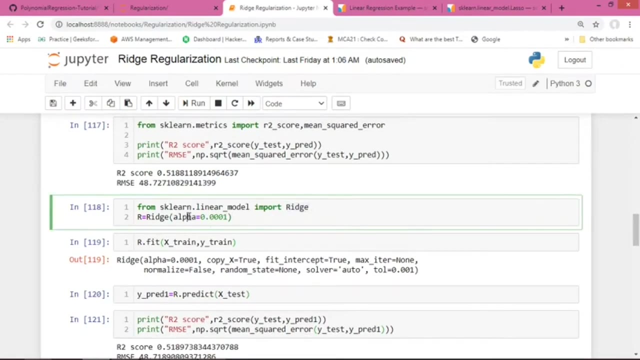 So apparently, the model is giving around 51% accuracy And the root mean square error is 48%. Now what I have done is the same thing with ridge regression. So what you have to do is you have to import this class ridge, And in ridge there is this hyperparameter alpha. 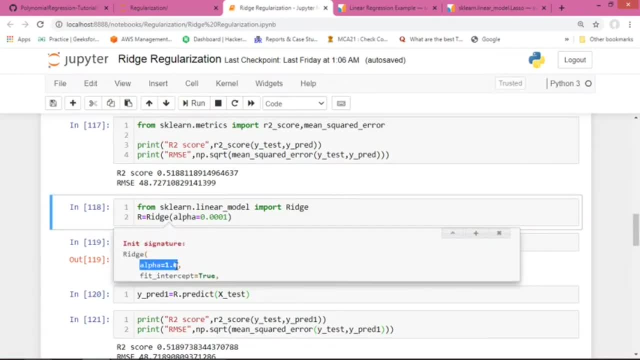 Which is basically the lambda which I have discussed in the last video. So its value is by default 1. So you can use 2-3 strategies. The first strategy is to try for different values again and again. The second strategy is to use cross validation. Use grid search, CV. 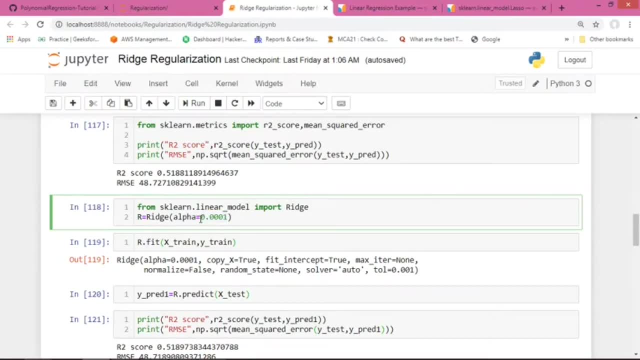 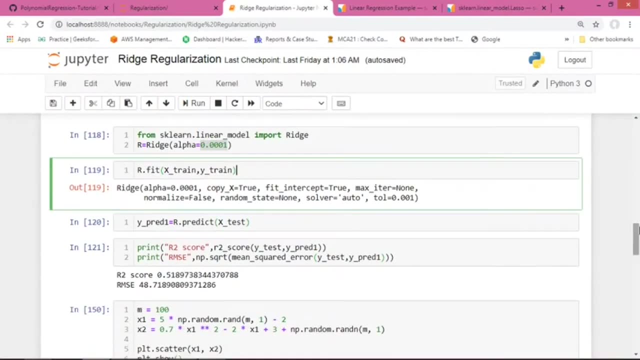 So I have tried with 2-3 values And now I have kept its value as 0.0001. And then I have trained the model On the same values And here I have calculated wipe-read 1 On the same test data set, And here you can see the accuracy score is exactly same. 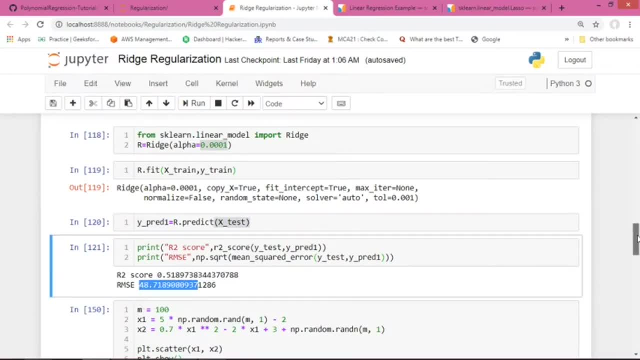 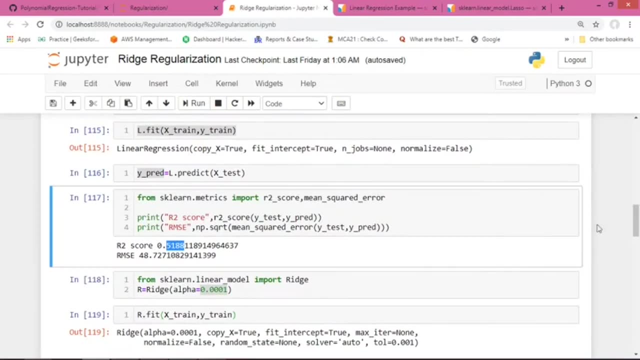 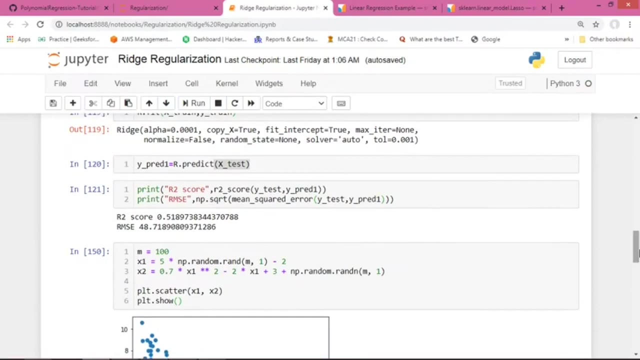 Almost same. actually, 0.5189 is coming here And I guess it is coming up here Just one second. Yeah, 0.5189 Like slightly better performing ridge regression Over linear regression on newer data sets. So, to be honest, there is not much upgrade. 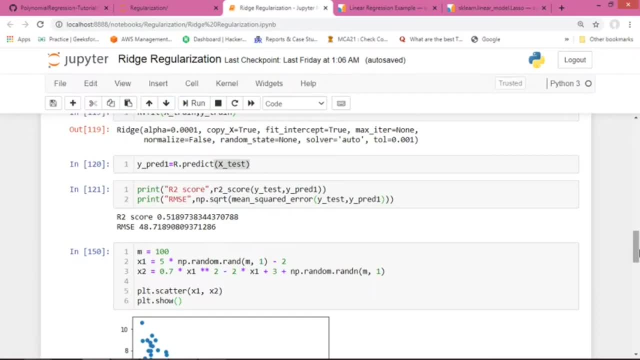 But the whole idea is that This model is slightly less complex In comparison to the previous one. Okay, So there is not much difference, But if you use lasso regression, You would see a significant improvement in R2 score When you are dealing with newer data sets. Okay, 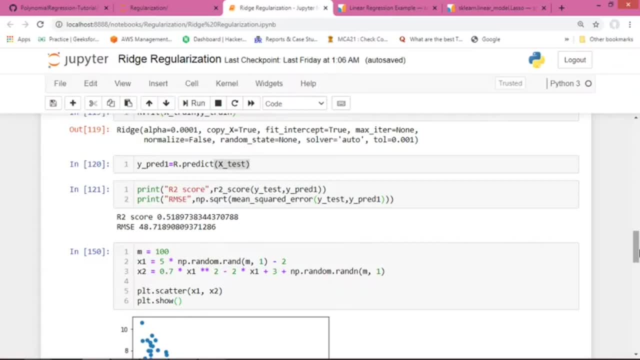 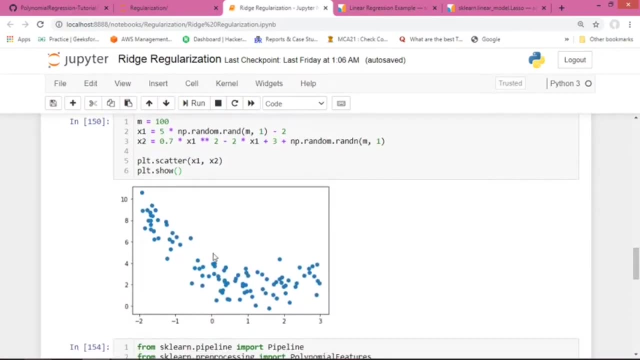 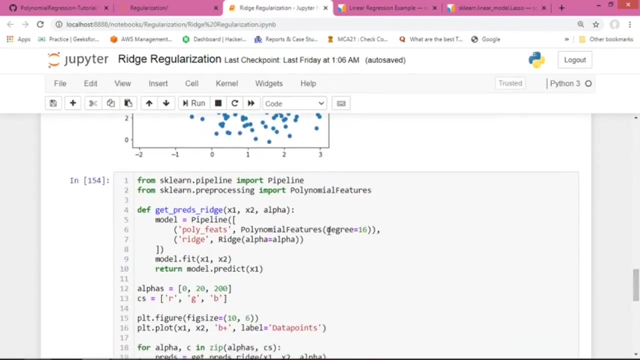 And after that what I did. I just wanted to show you How overfitting and underfitting is done In the case of ridge regression, So I generated a data set Which is kind of non-linear. Okay, And then what I did? On top of this, I applied degree 16, polynomial regression. 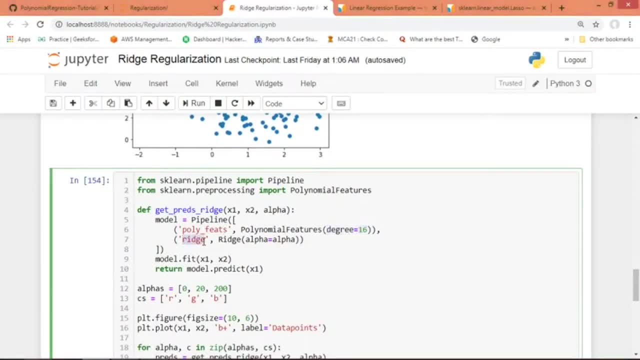 Okay, And this time I did not solve it with linear regression, I tried to solve it with ridge regression And I tried three values of alpha: 0, 20 and 200. Okay, So 0 means that ridge regression will not actually apply, Because as you multiply lambda. 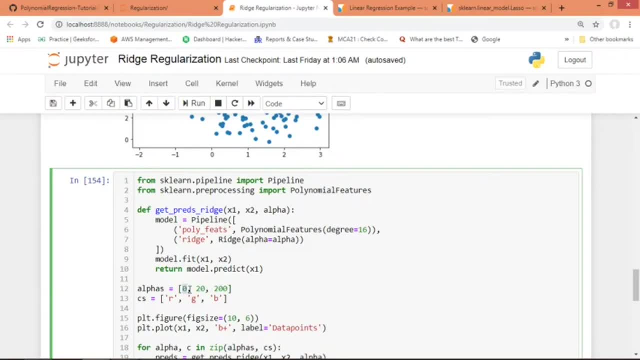 All the slopes will become 0 And your model will perform exactly like linear regression. Right Then 20 is like the optimum value, Where you will see the best curve, And in 200 it will start to underfitting Because you are very much Reducing the weight of your slopes.